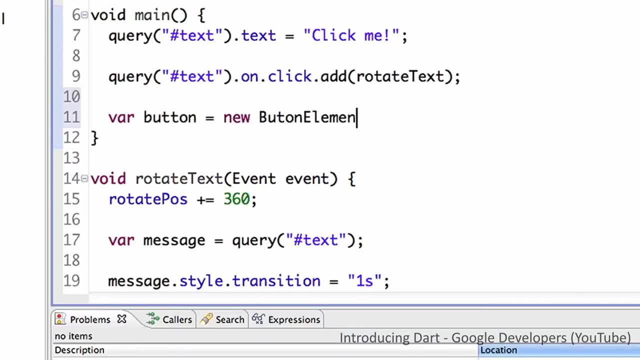 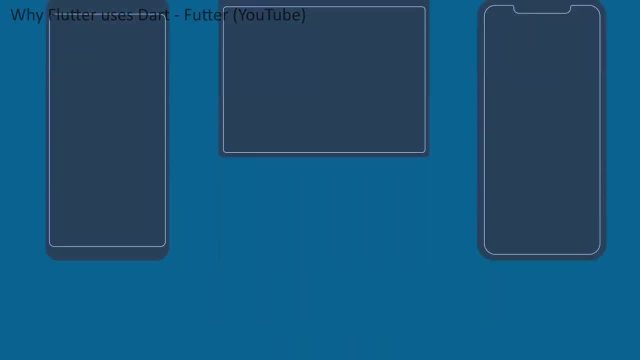 C-style syntax and garbage collection, as well as being object-oriented. Interestingly enough, Dart can actually compile to JavaScript in order to support running on popular web browsers For my mobile app developers out there. you may have heard of Dart, which is a 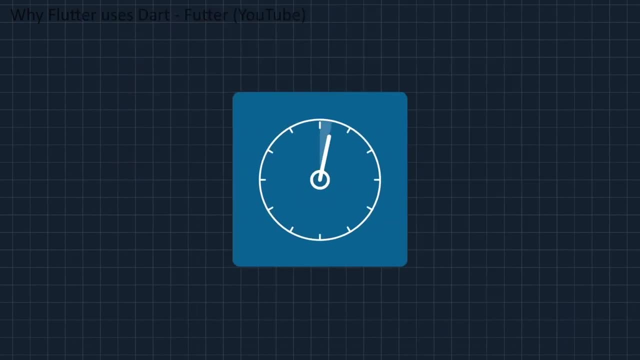 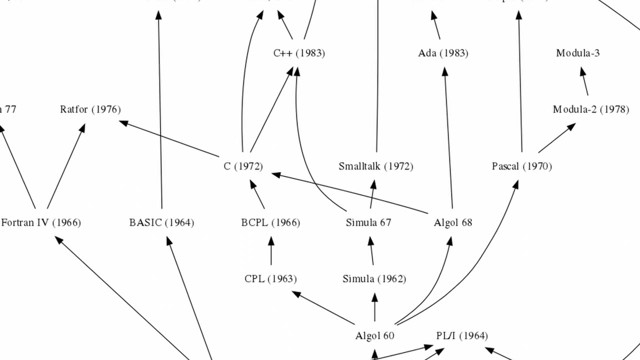 well-known programming language that was also released by Google and actually written in Dart. If we are talking about family trees, Dart is yet another child of the ALGOL programming language family, alongside its older siblings C and Java, Now for one of the most requested programming. 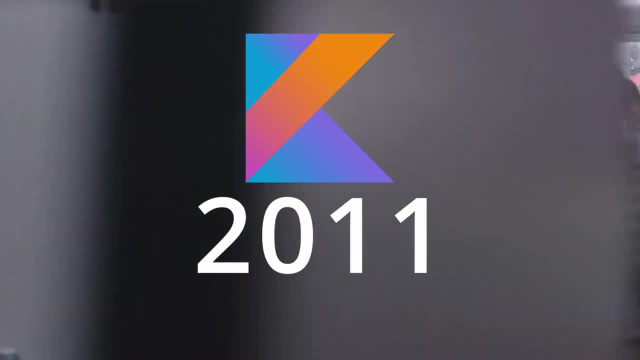 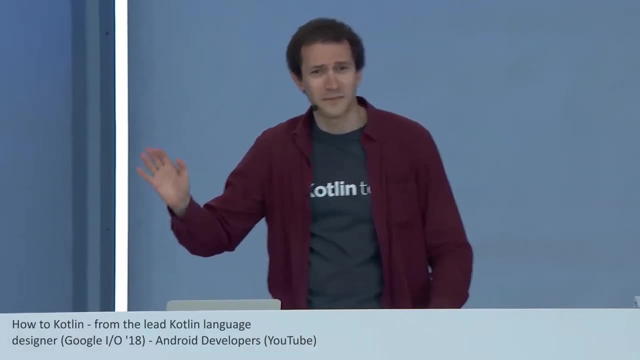 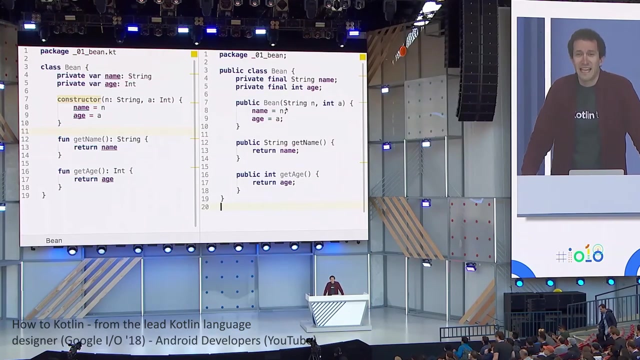 languages. Also in 2011,, while Dart was darting around app platforms, the programming language Kotlin was released by the Czech software development company JetBrains. Kotlin is more of a general-purpose type programming language, but primarily used in Android app development alongside Java. Kotlin and Java are actually very much intertwined. 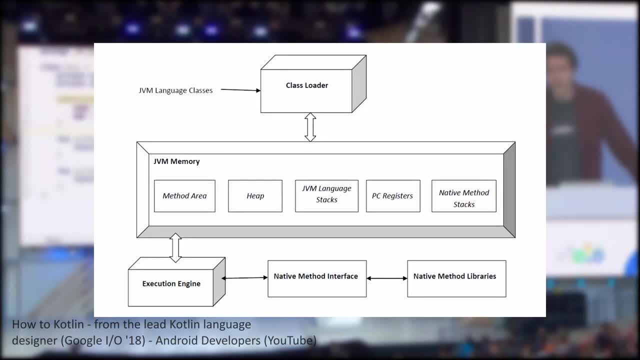 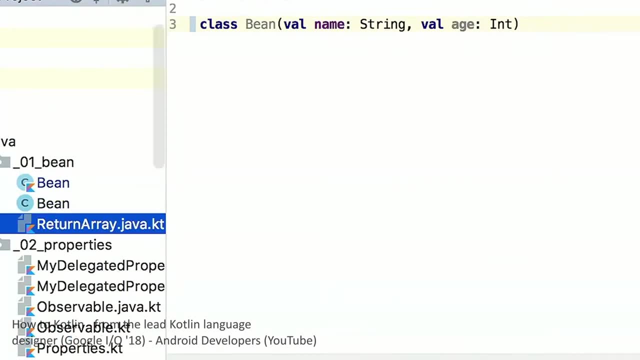 as Kotlin is primarily targeted to the JVM or the Java Virtual Machine, to compile Java code regardless of the device, as well as work in conjunction with Java code, and Kotlin even relies on the Java standard library. Additionally, it's not uncommon to mix. 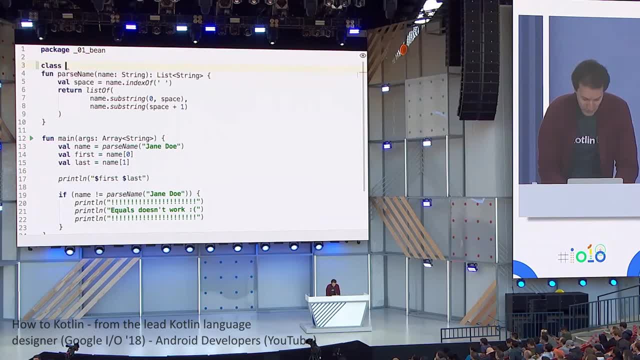 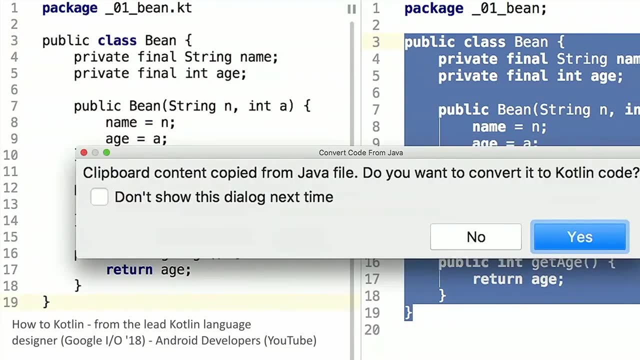 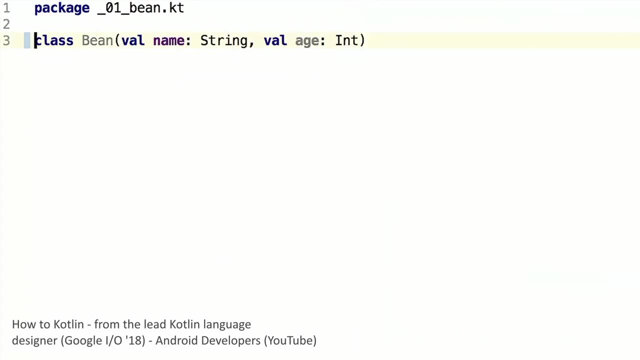 both Kotlin and Java together in the same project, but you can't quite use their syntax interchangeably yet, So it will use the Java to Kotlin converter built into the IDE and do it for me. So, boom there, it is A single line. that's actually all you needed. 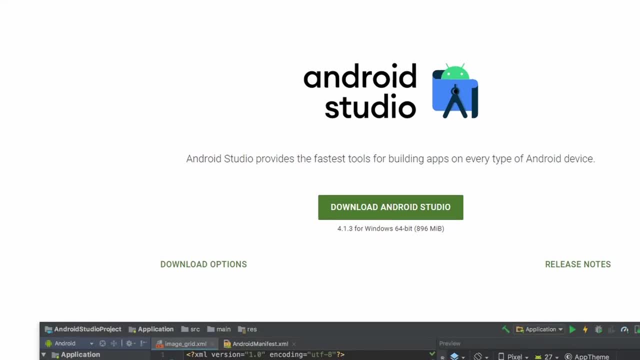 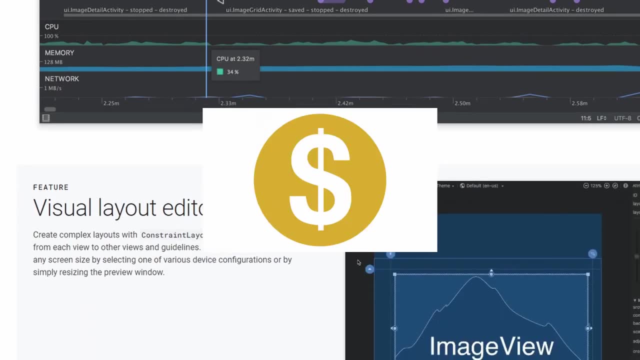 to declare one class, two properties. If you want to get started developing some Android apps and dive deeper into Kotlin or Java, you can download Android Studio for free- this isn't an ad- and try your luck at becoming the next app millionaire, Moving to 2012,. 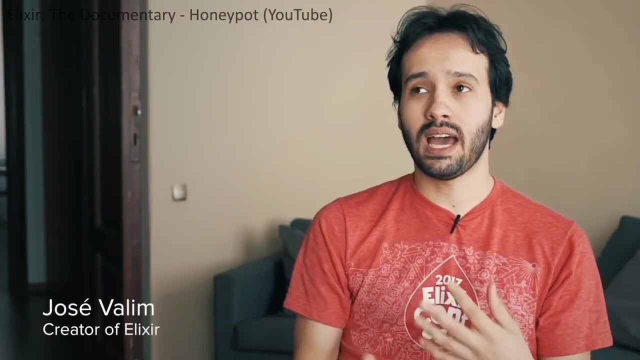 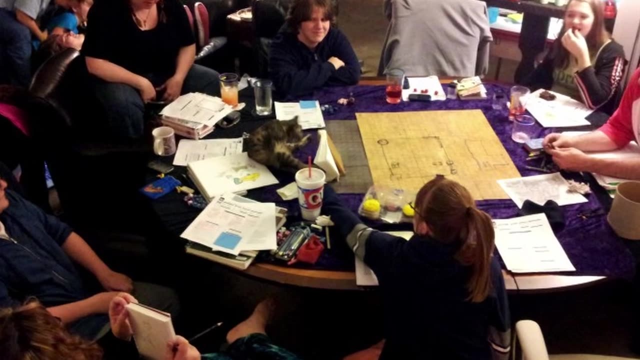 the programming language Elixir was released, originally created by Jose Vallam. Now, this isn't regular magic Elixir that you might find at your bi-weekly Friday Night Dungeon and Dragon sessions. Elixir is another general purpose and functional programming language, but mainly focused on 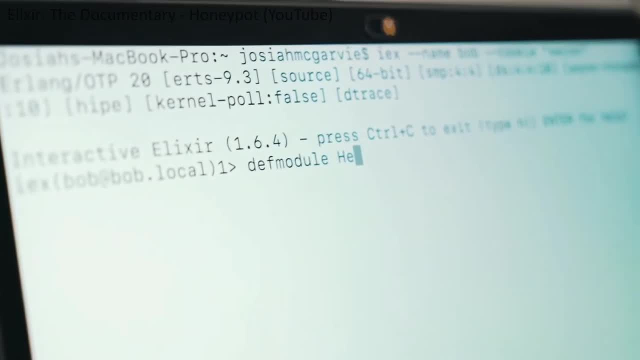 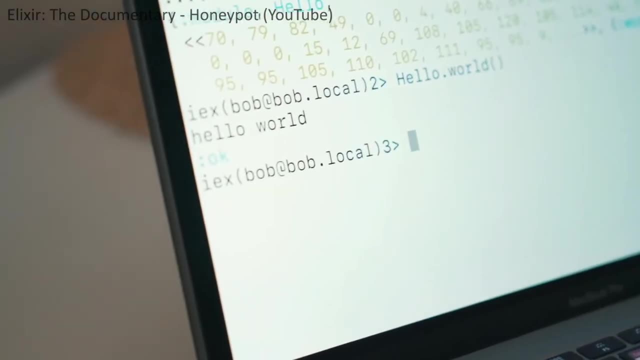 handling large amounts of data. It targets the Beam Virtual Machine, which is a part of the Erlang runtime system. Vallam envisioned Elixir because he wanted better productivity and extensibility whilst keeping the benefits of the Erlang ecosystem compatibility. So one of the big 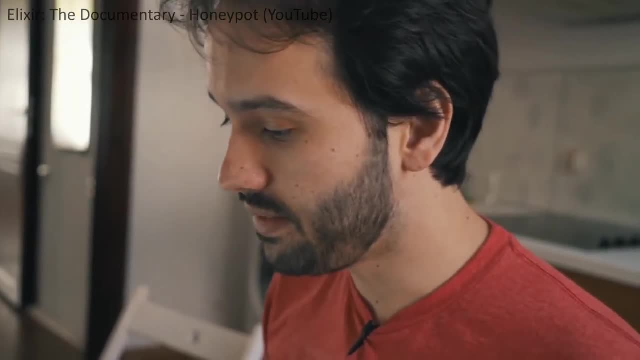 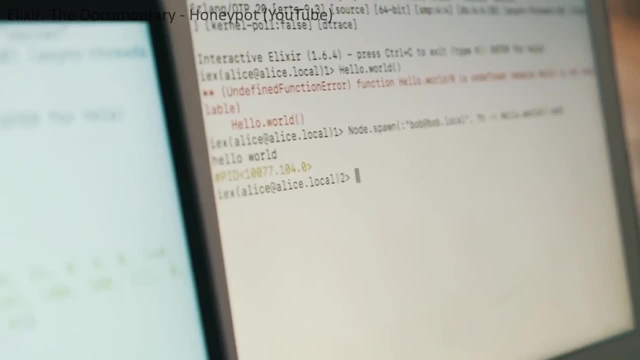 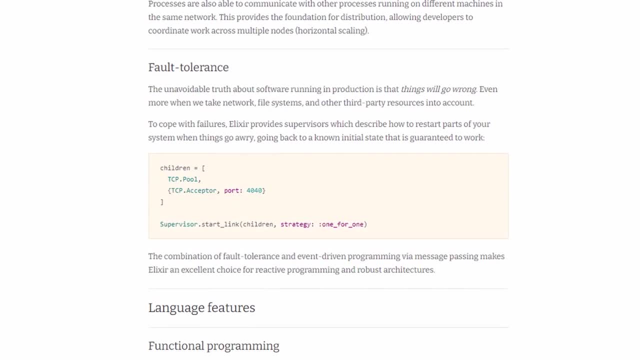 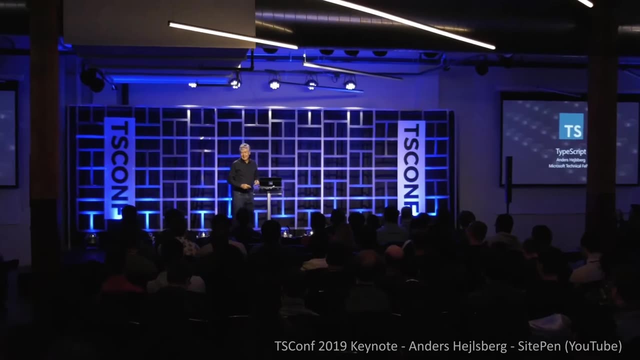 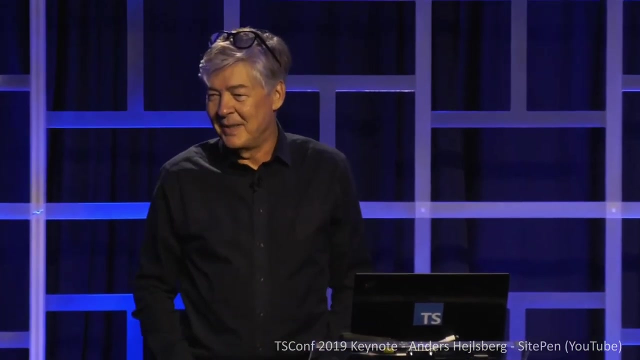 creating Elixir. One interesting bit about Elixir is its fault tolerance protocol that basically utilizes programmatic supervisors to monitor and suggest restarts when encountering a problem. Fellows over at Microsoft, specifically, Anders Helzberg, released TypeScript in 2012 and had influence from C-sharp, Java and Javascript. TypeScript was created as a 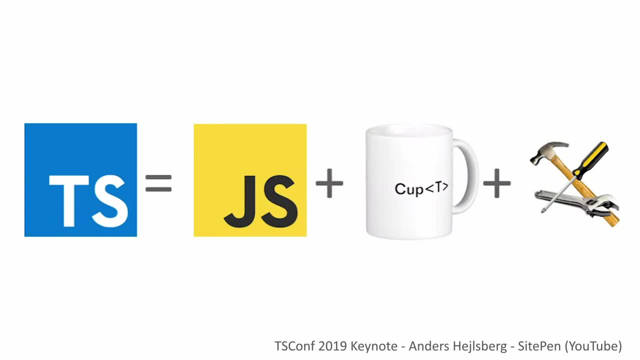 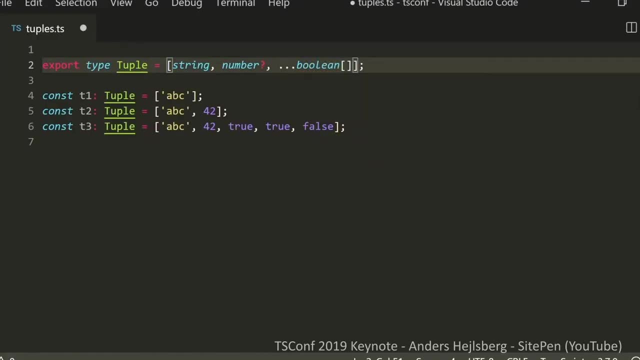 syntactical superset of Javascript, which basically just means it encapsulates all all of the syntax of javascript while adding, more most notably, static type definitions. therefore, definitionally wise, all javascript files are technically typescript files. it was also birthed out of some of the downsides of javascript, specifically large-scale software development. 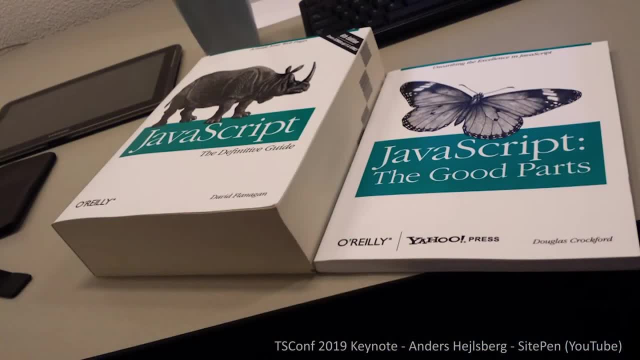 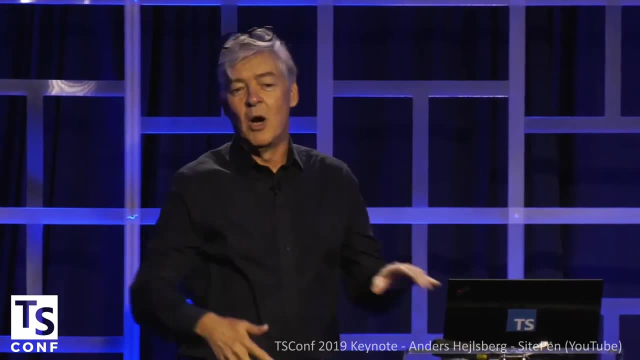 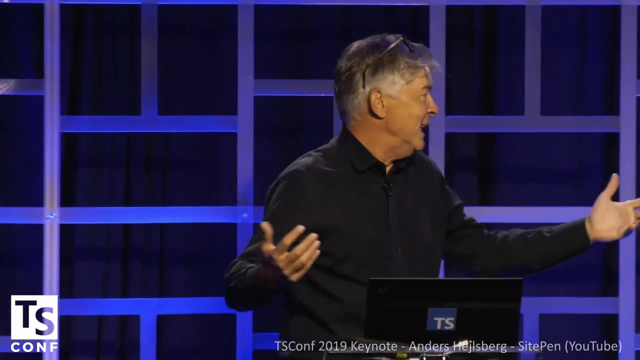 this in a nutshell is: is why we're here, right? um, javascript is a great language, but it has issues, uh, and, and it needs tooling if you want it to scale. and really, that was sort of like the, the insight that that we- and not just we, but many uh- had, you know, years and years ago, and that was 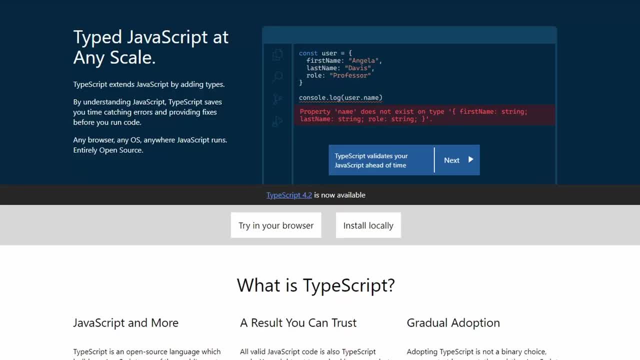 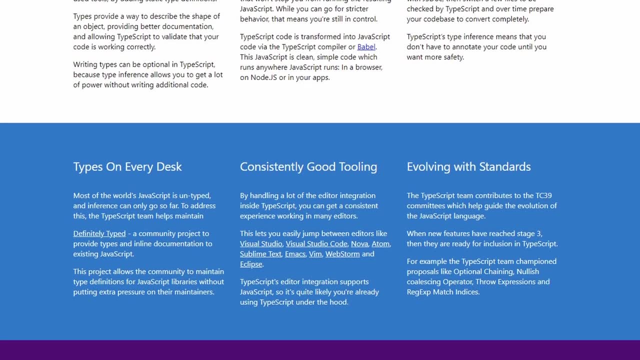 in a sense, what, what? what got us started? typescript is open source, if you want to go poke around, and similar to dart. typescript can compile to javascript and features a pretty unique definition file feature that sort of acts like a c plus plus header file. typescript 4.0 was recently released. 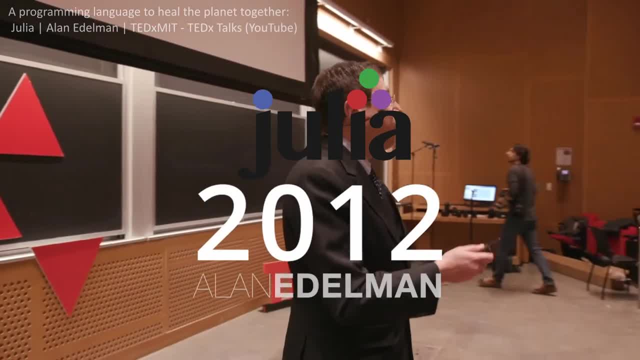 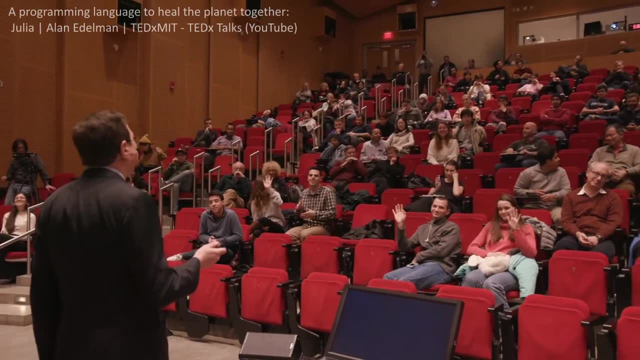 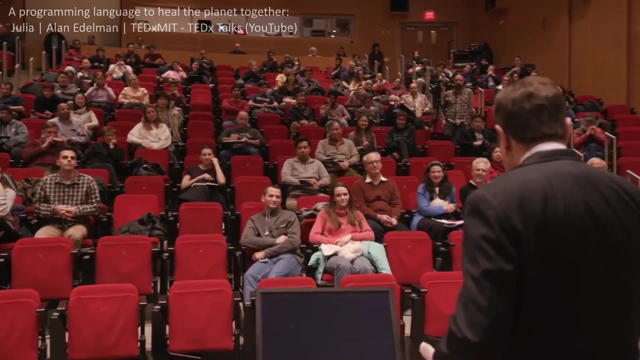 on august 20th 2020.. around the same time, in 2012, the dynamic programming language, julia, was released. similar to some other math and math mathematical programming languages, like matlab, julia really shines when it comes to numbers and general computational science problems. i'm a co-founder, co-inventor of a programming language. 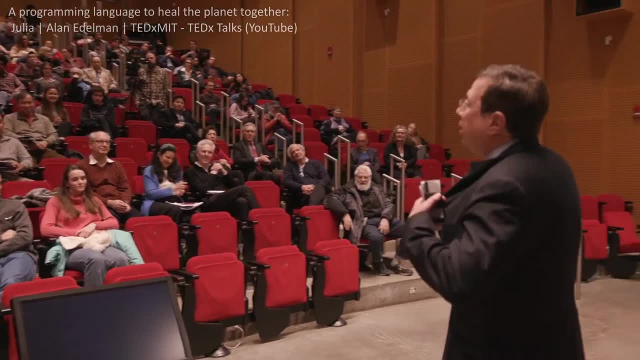 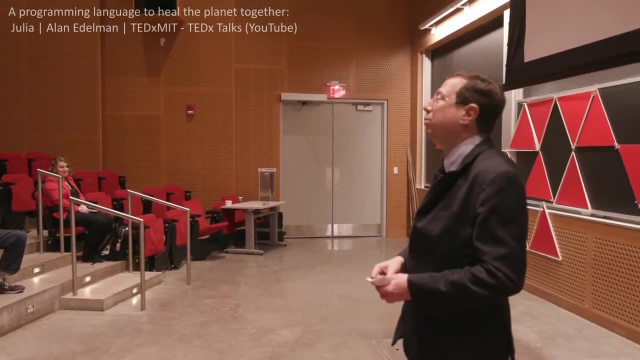 known as julia. perhaps some of you have used it, and this language is become increasingly popular for all of the various kinds of models that will be coming up in the various talks today: the climate models, the economic models, the various political models and so forth. julia- 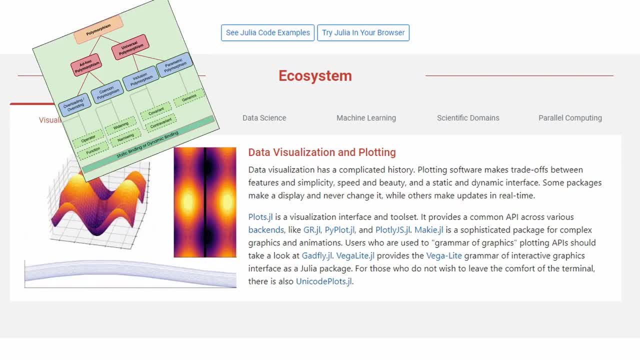 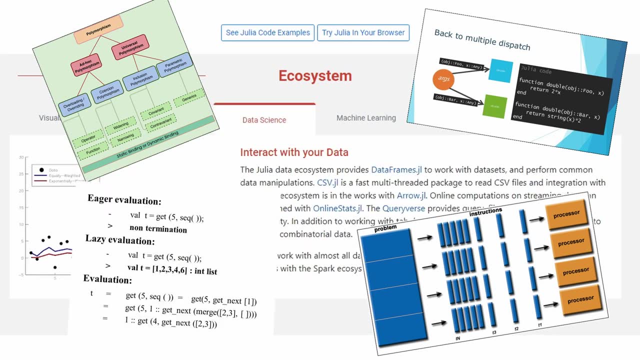 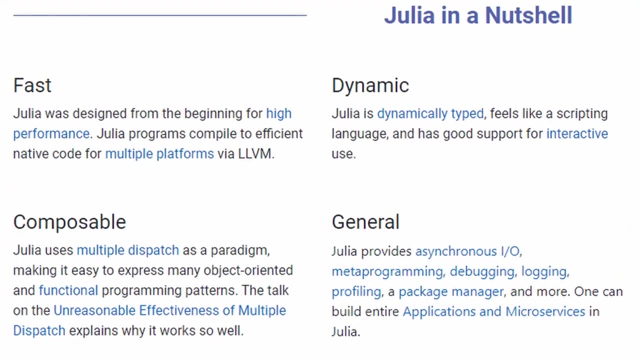 features a lot of big science words like parametric, polymorphism, multiple dispatch paradigms, parallel and distributed computing, eager evaluation and some other math science stuff. julia utilizes a just-in-time compiler which compiles all julia code to machine code before actually executing it. jeff bexenson, stefan karpinski, viral b shaw. and alan edelman were the main crew to formulate julia. you may be asking yourself where they got that name. maybe it was one of their beloved partners or children, perhaps a cherished grandmother or a friend? well, no, they just liked the name julia. now, if you want to be an investment banker, you might. 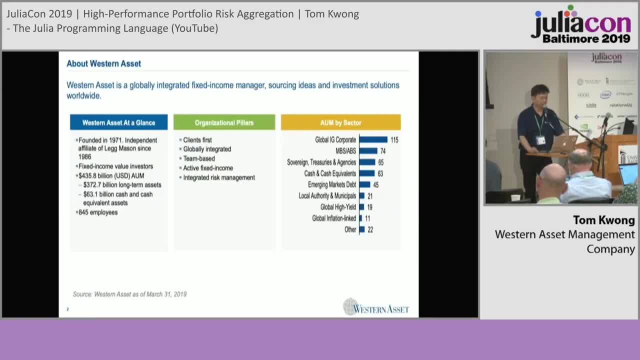 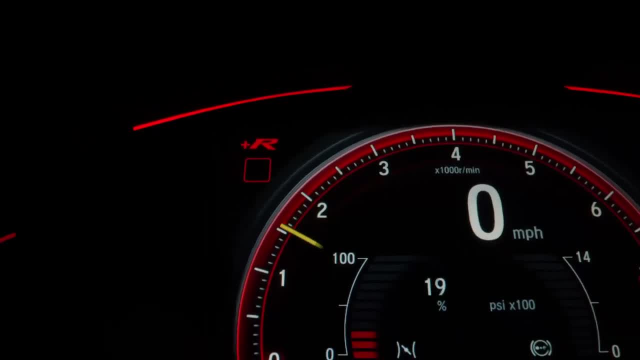 want to pick up julia as a side project, as it was used at both blackrock for time series analytics and the federal reserve bank of new york to make models of the us economy which, according to them, was 10 times as fast as the matlab counterpart. that's right. take that matlab, making me look a. 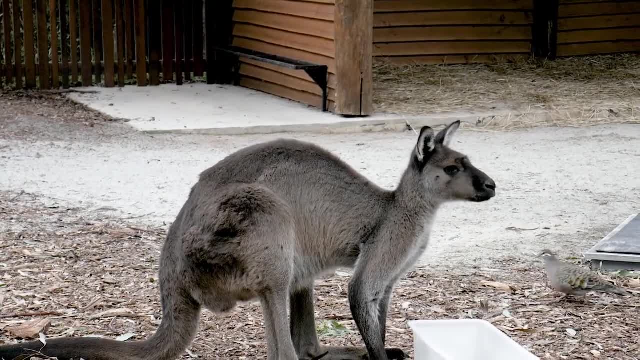 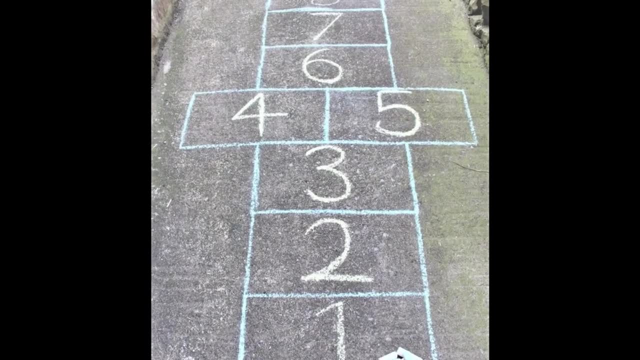 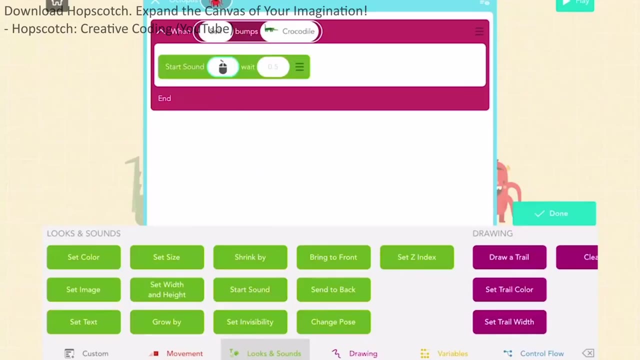 matrix documentation to finish my math homework. now we are going to hop our way over to hopscotch, released in 2013 by hopscotch technologies, the children's game it gets its name from. hopscotch is a visual programming language specifically designed for young and new programmers. its ui allows for dragging and 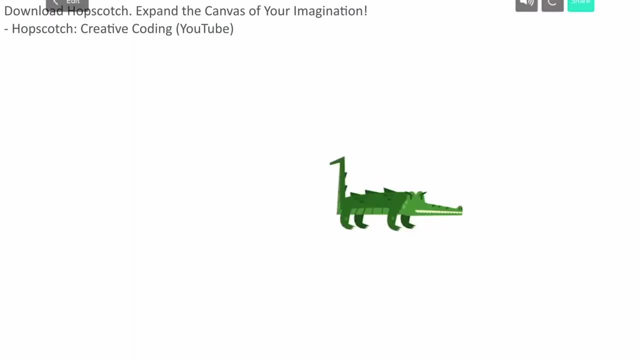 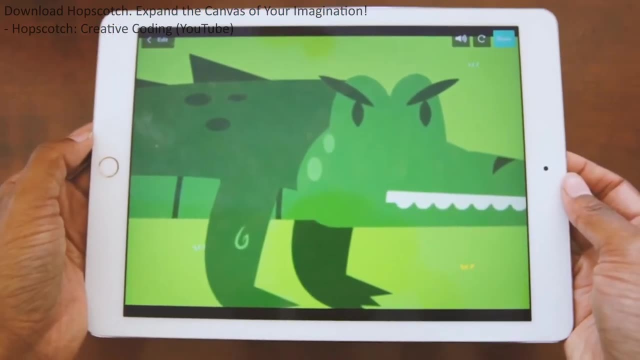 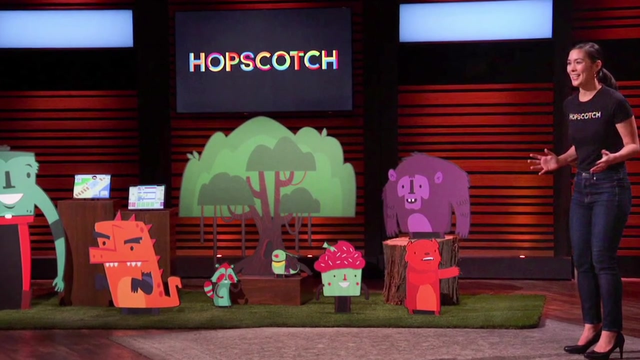 dropping code blocks and scripts to foster early education in programming patterns and paradigms. but since its focus is fairly narrow, it's not really used in any serious computation or applications. plus, the way you actually utilize hopscotch is primarily through their ios app was also featured on shark tank. so, uh, invest while you can. in 2013, we get cuneiform, not. 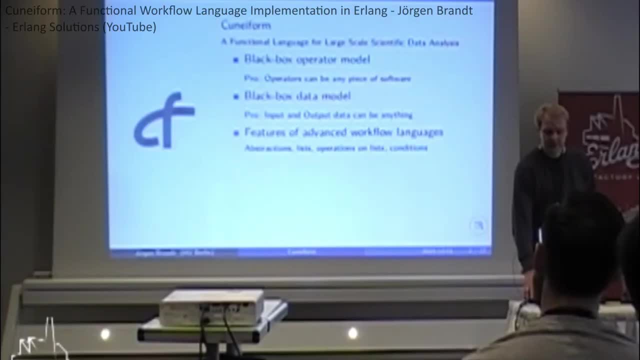 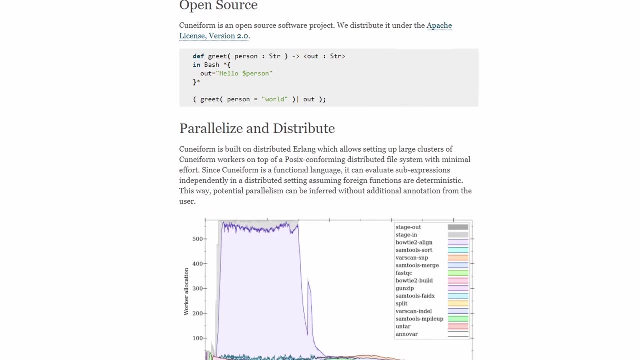 this, but this created by jorgen brandt. the original cuneiform was open source, and so was this one specifically targeted at large volume scientific data analytics as well as parallel computing. so what we're facing today in the field of bioinformatics, and especially in next, 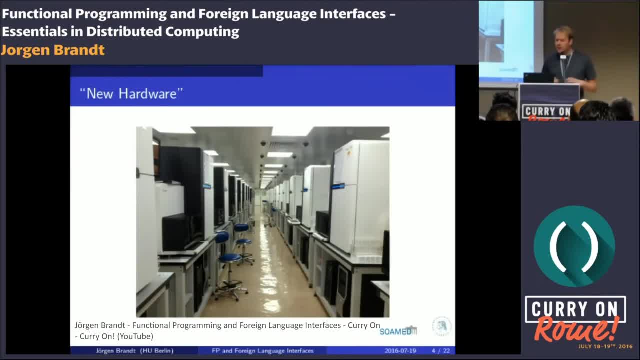 generation sequencing is that there's coming up a new kind of hardware which is capable of producing data extremely fast. also, you can operate it very, very well in parallel. it's natural to say that if we can generate this data in parallel, we also have to analyze it, since cuneiform is 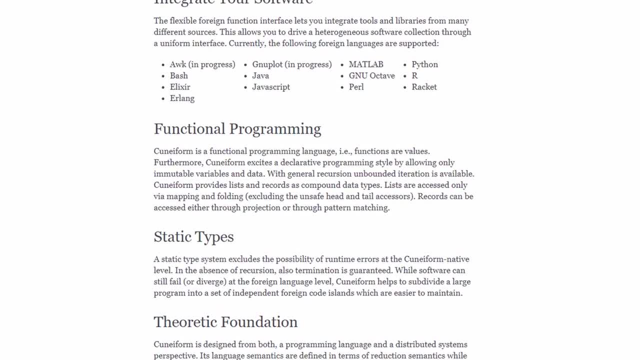 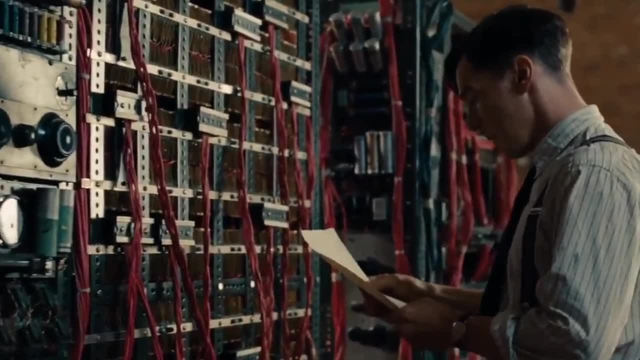 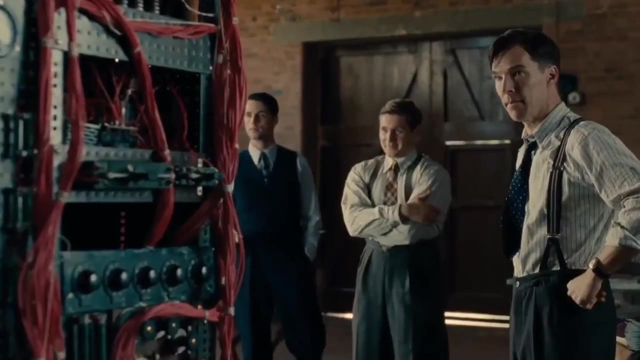 primarily a programming language for mathematics and scientific computation. it's a functional programming language and, interestingly enough, cuneiform is also turing complete. now i still get confused on what being turing complete actually means, but it basically means that it can simulate any turing machine- and a turing machine is a whole other history video- but without getting too deep. 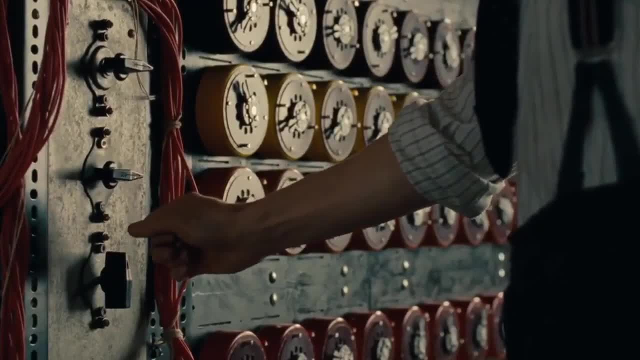 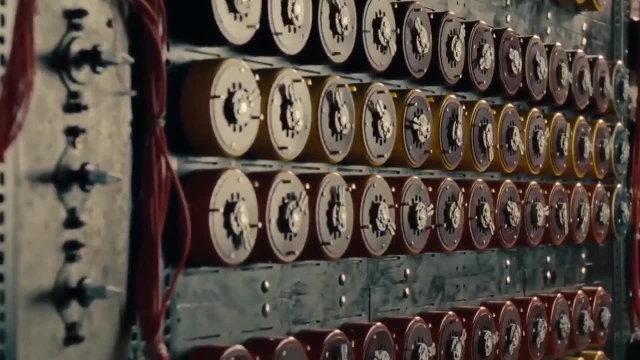 essentially it's a theoretical mathematical machine that uses a tape and rule sets to do stuff. so throw it back to the early bronze era and take a dip into the cuneiform programming language. now we are going to skip ahead a bit to 2014. while you were listening to steal my girl by one direction- and i know you were- 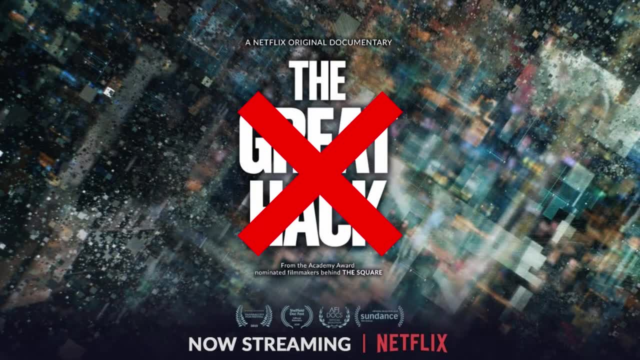 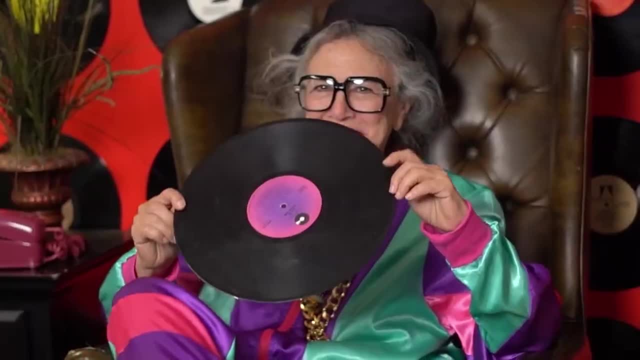 facebook released hack, not the netflix documentary, the great hack and at this point that name sort of aged poorly hack and i'm not making this up. it targets the hip-hop virtual machine. maybe the developers were listening to 2014 music while writing it. ultimately, hack is: 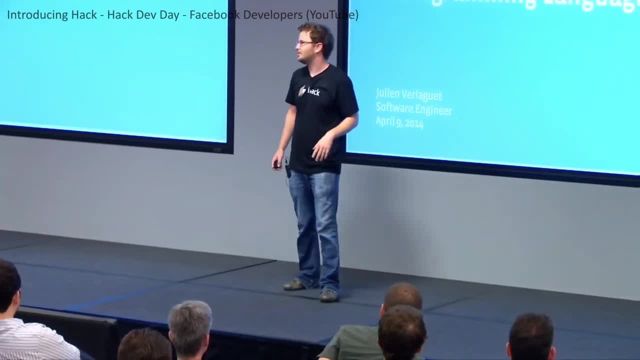 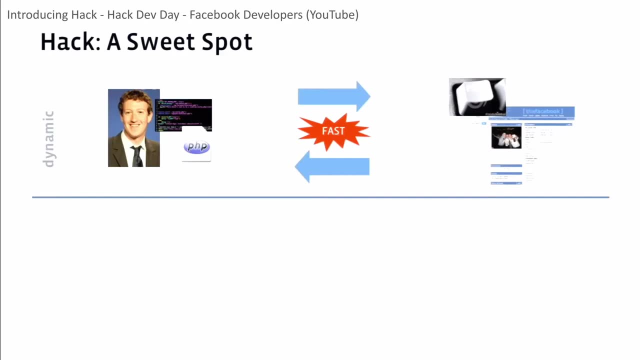 a variant of the popularly means on web development language, php. talking about php and um. so i picked a random php developer- you might have recognized him- and he was trying to build something. right back then in 2004, he was trying to build something called the facebook. 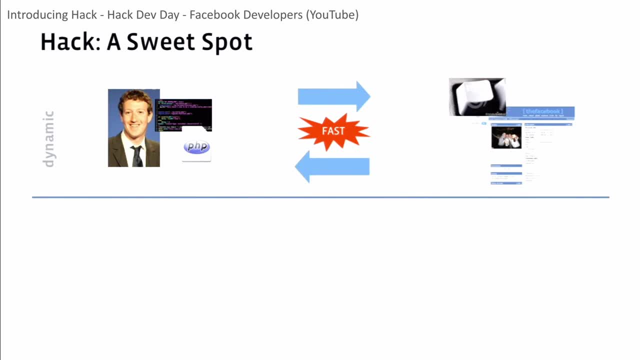 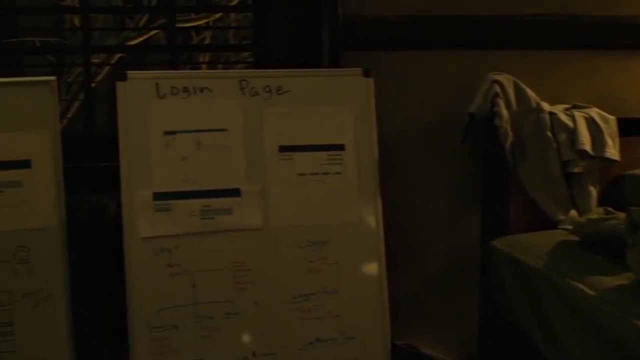 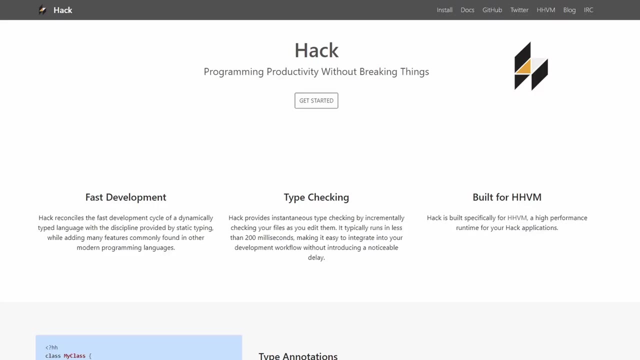 and he picked a technology to do that. that was php, and we think that it has been a really good choice. before releasing it to the public, facebook integrated hack into it. facebook in order to stress test its web development and large scale capabilities. hack supports both dynamic and static typing and even has instantaneous type checking periodically. 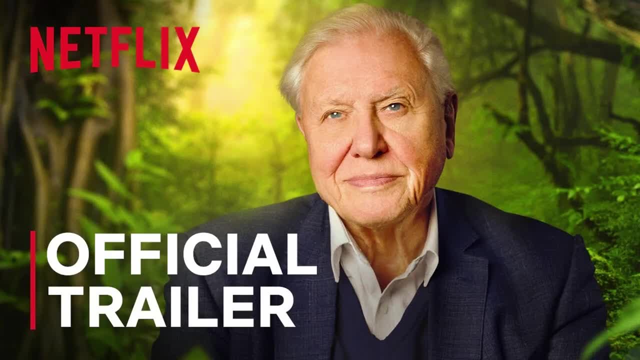 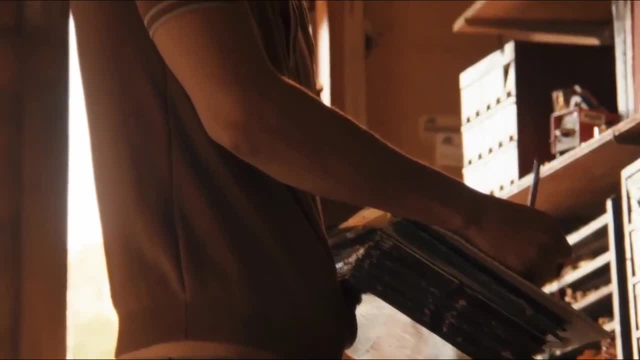 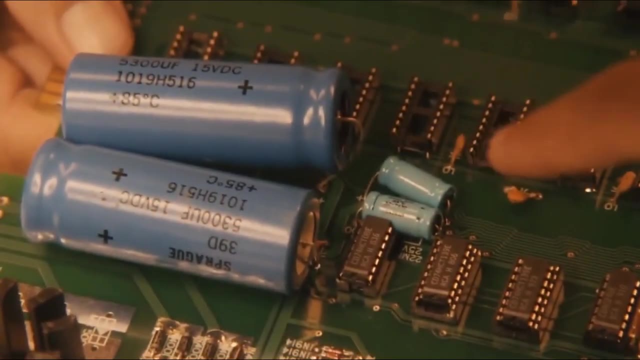 checking files while they're being edited. all right, for this next one, we're gonna do a british slash australian narration voice, so uh, buckle up in a classic tech rivalry. swift was also released in 2014 by the big lads and lasses over at apple. now i've covered swift before, so i'll keep it. 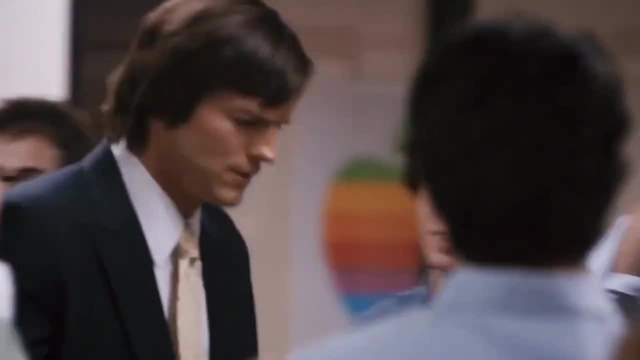 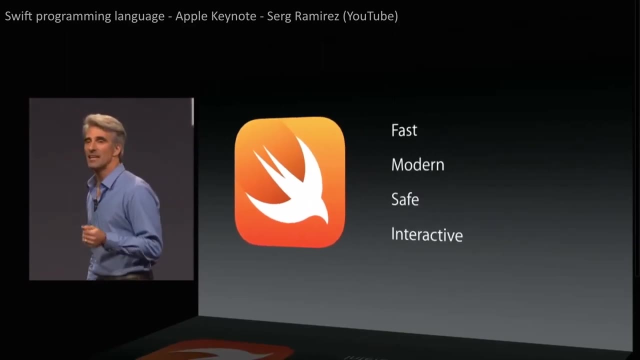 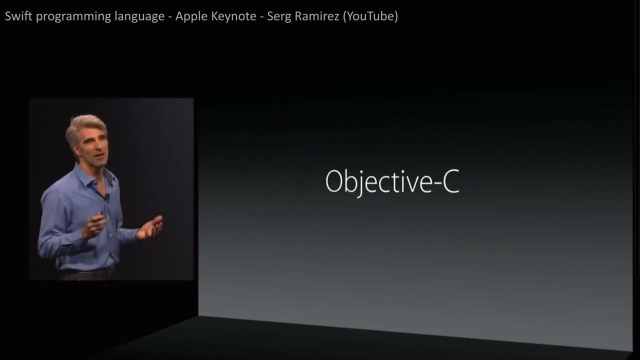 brief. prior to swift, objective c was the primary program that was released by the big lads and lasses programming language in many apple products. but just like removing the headphone jack, swift was designed to replace the older objective c and introduce more modern programming features. objective c has served us so well for 20 years. we absolutely love it, but we had to ask ourselves the 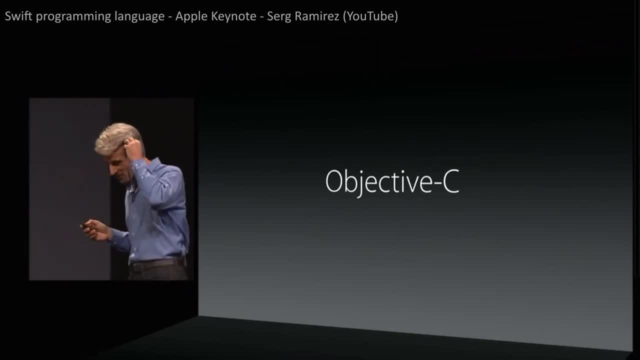 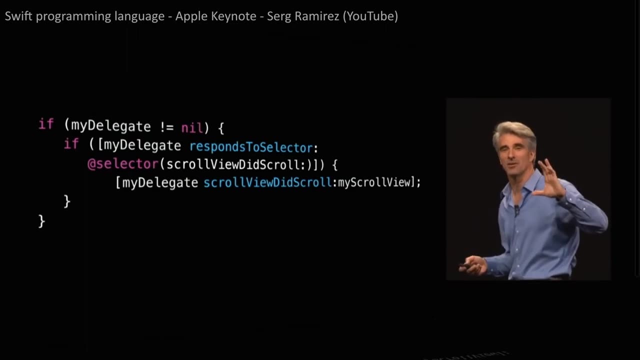 question: what would it be like if we had objective c without the baggage of c? since so much of the existing code at apple was written in objective c, they couldn't just do a hard swap. so swift was designed to interrupt the programming language in many apple products. swift was designed to 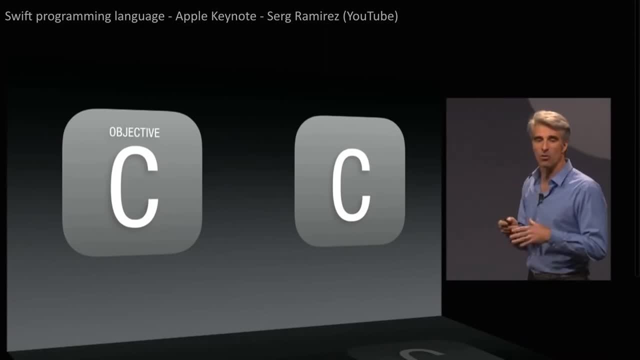 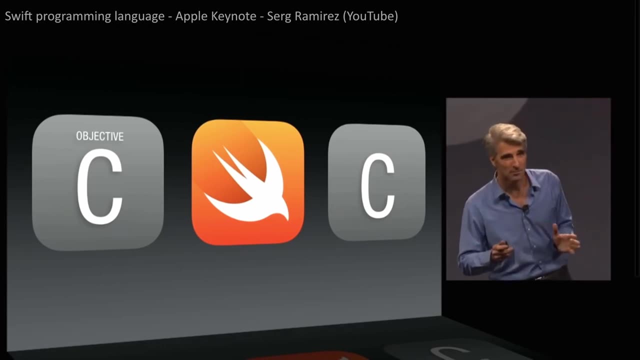 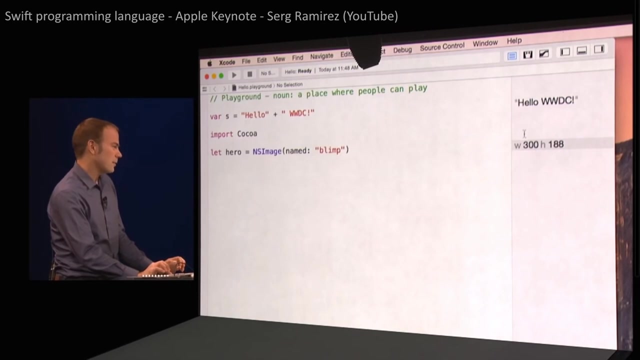 operate and coexist with objective c code and specifically within apple products. swift utilizes the objective c runtime library, which ultimately means that within a single program, swift, objective c and even c can operate. swift is the main programming language for writing ios applications and, from personal experience, it's quite easy to read and pick up and one interesting. 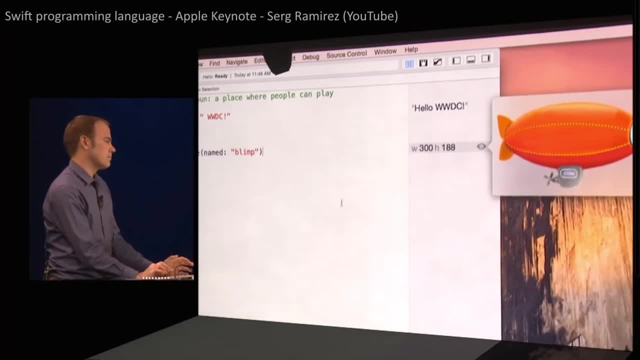 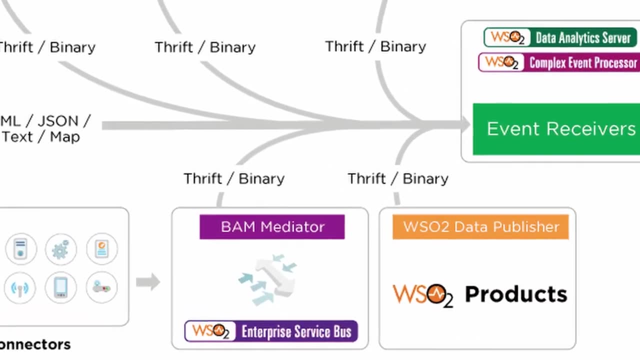 point, swift doesn't reveal unsafe accesses like pointers, to avoid those pesky null pointers. to pick up the piece a little bit, we're going to move to ballerina in 2017.. originally provided by the open source group wso2 and still remaining open source, ballerina was formulated. 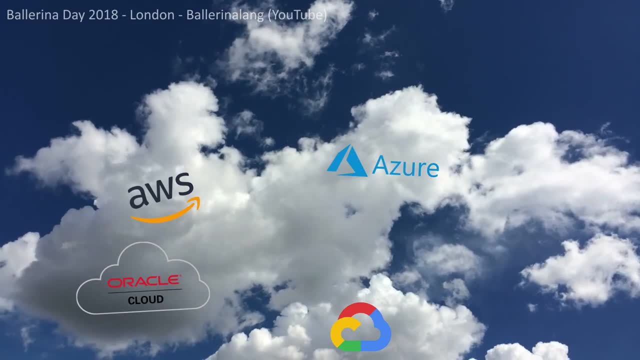 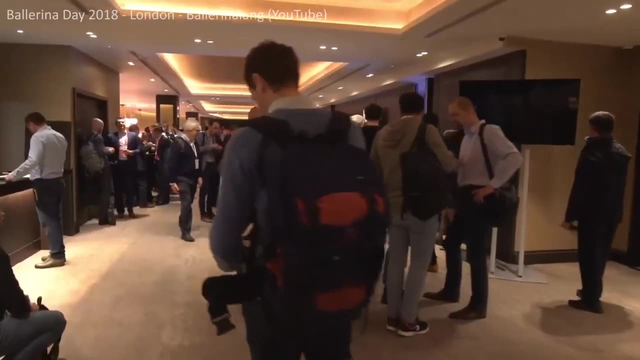 with the growth of cloud programmers in mind. i mean, look at how many clouds are out there. many of its features are focused on cloud native development specifically. a very handy aspect of ballerina is that for every ballerina program, a corresponding sequence diagram is also created. 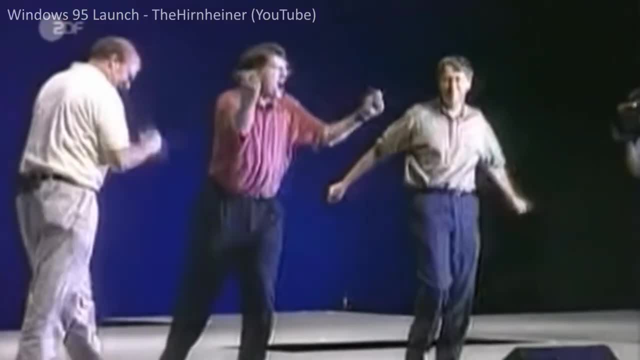 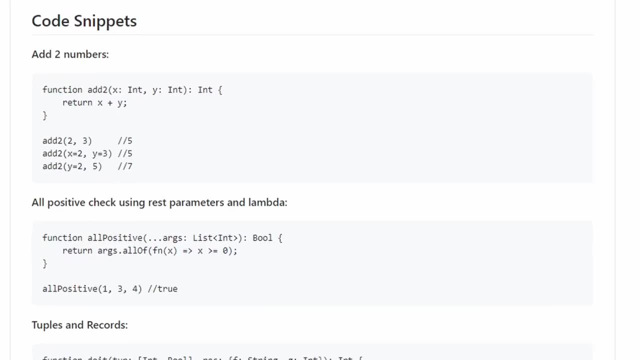 to show software interactions. now for another microsoft banger. only two short years ago, bosk was released by mark marin in conjunction with microsoft. another open source language. bosk was the first to come out of the box game which included open source programming in the form of. 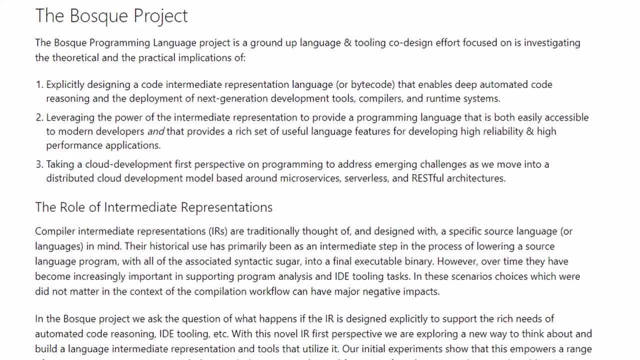 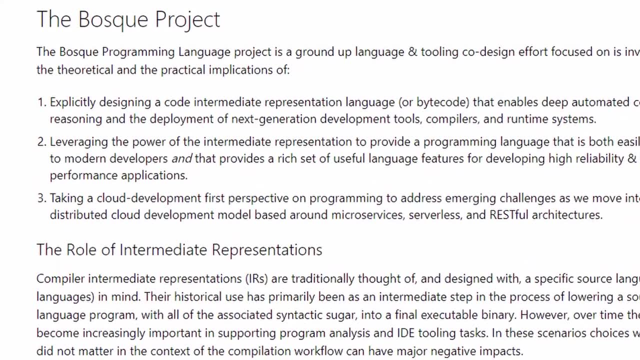 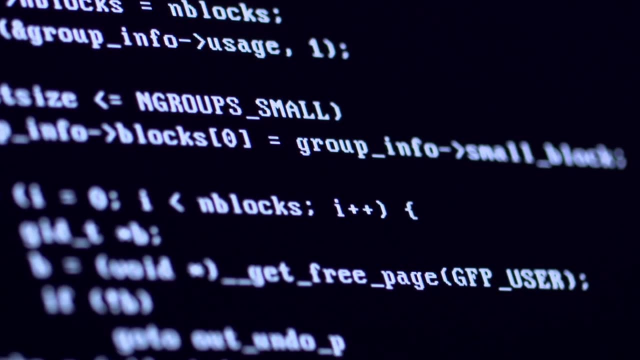 an on-demand version of the library program and it's a great way for beginners to dig deeper into different aspects of typescript combined with the programming semantics of javascript. osc is currently still in development to research and enable automated code reasoning, intermediate representation for easy and highly reliable and well-optimized programs, as well as honing in on 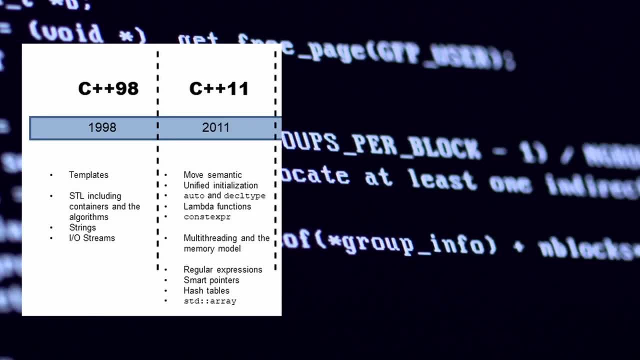 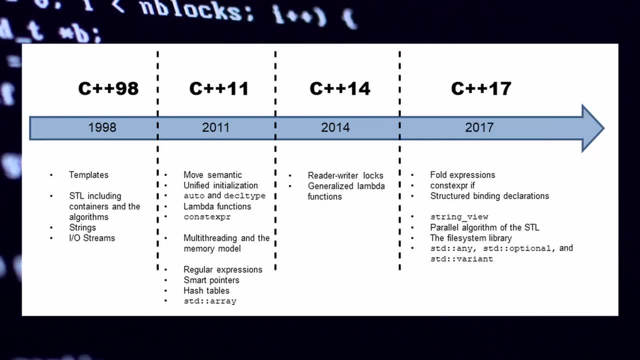 cloud-centric development and, as of march 2021, bosk is on the road to version 1.0. now for some notable throwbacks of popular programming languages that got some updates. c plus plus 11 was released. same with C++70.. Its older brother C's most recent iteration was C18, released in 2018,. 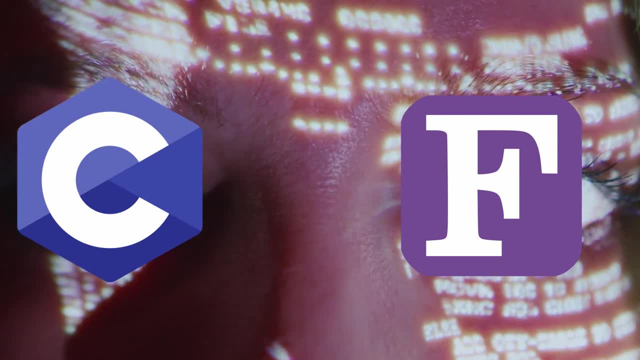 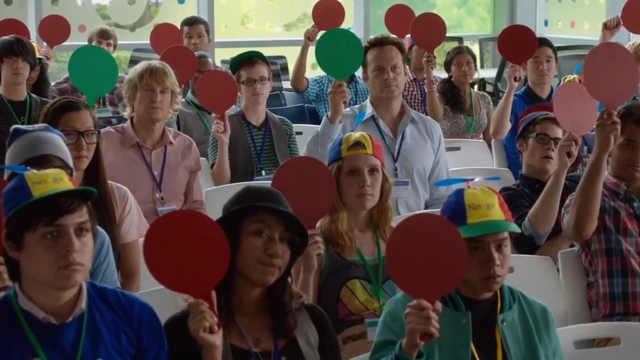 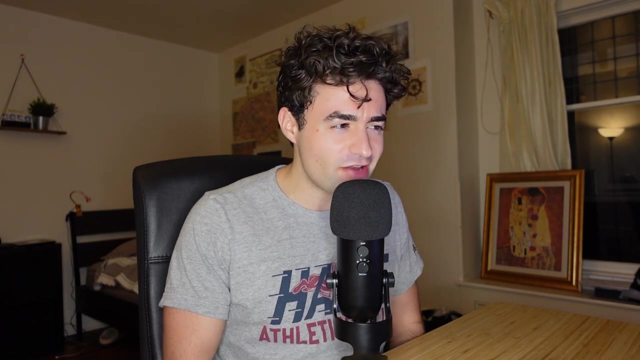 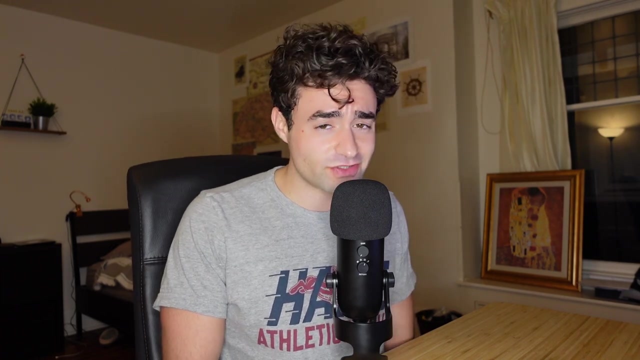 and even Fortran saw some nice updates with Fortran 2018.. And that has been the brief history of programming languages in the 2010s. I hope you guys all liked that video and found it, you know, somewhat informative and hopefully my British narration voice wasn't too terrible. My name is Michael. I make college. 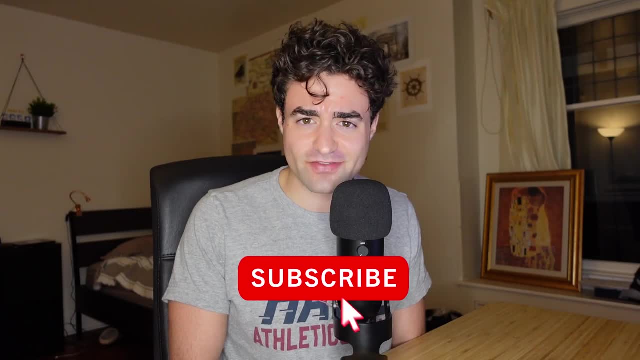 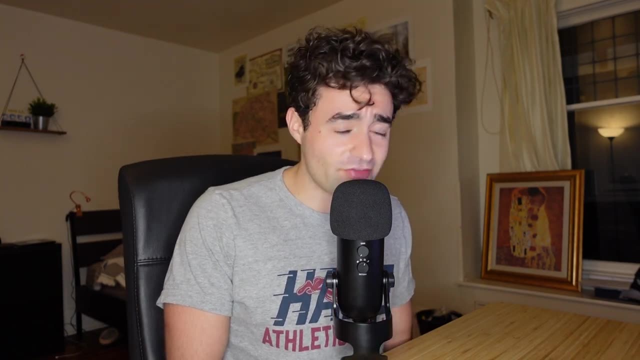 advice, career advice, tech, computer science videos. If any of those sound interesting to you, consider subscribing to the channel liking this video to help your boy out with the YouTube algorithm. And at the end of every video we do another Bad British Accent. Check out one of my. 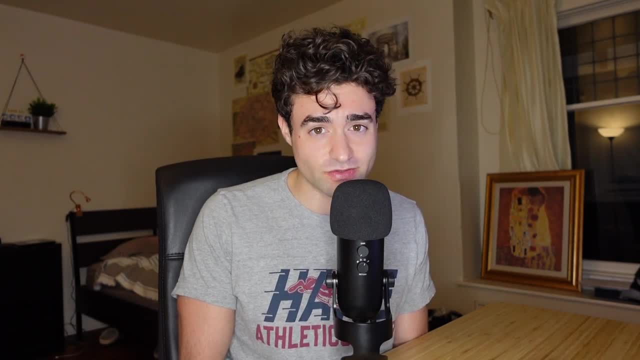 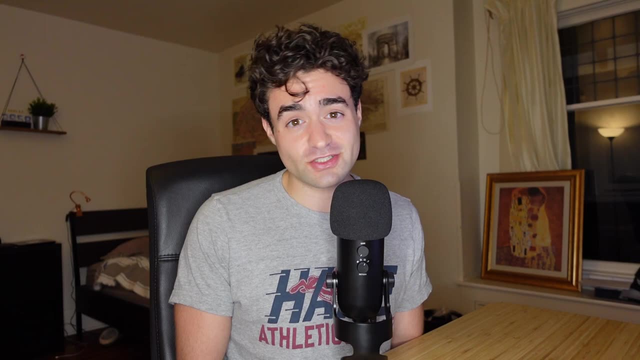 past videos and my past self would thank you dearly and check out one of my future videos and my future self would also thank you dearly. That's all from me. New backdrop: this time I changed rooms, So hopefully I put some fun stuff up there in the background, So